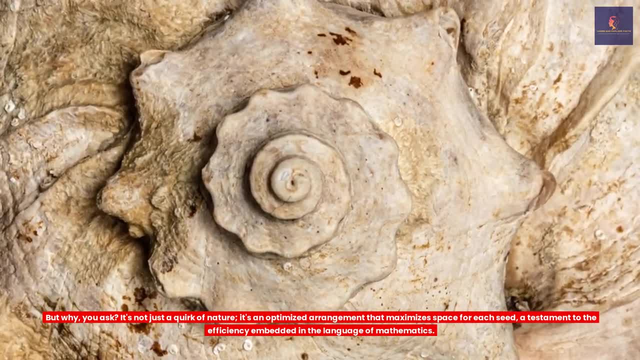 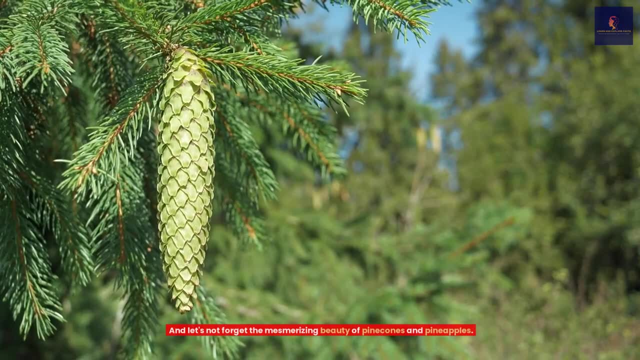 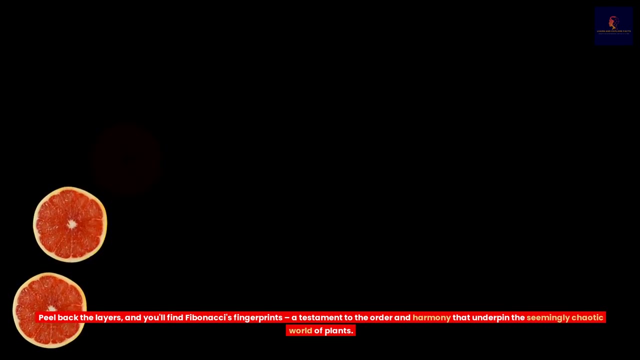 quirk of nature. it's an optimized arrangement that maximizes space for each seed. A testament to the efficiency embedded in the language of mathematics. And let's not forget the mesmerizing beauty of pine cones and pineapples. Peel back the layers and you'll find Fibonacci's fingerprints. 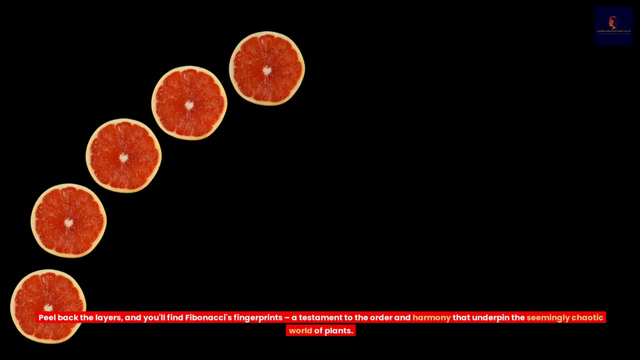 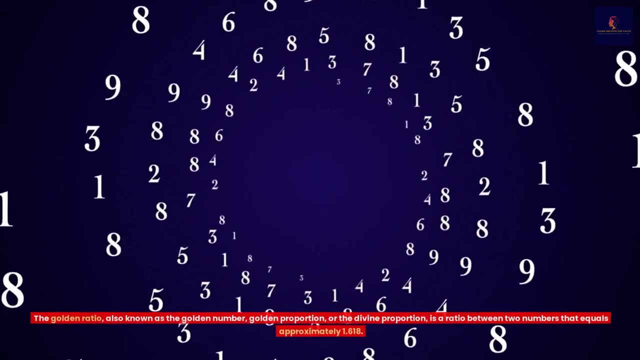 A testament to the order and harmony that underpin the seemingly chaotic world of plants. Now let's spotlight the enigmatic star of our show: the golden ratio. The golden ratio also known as the golden number, golden proportion or the divine proportion. 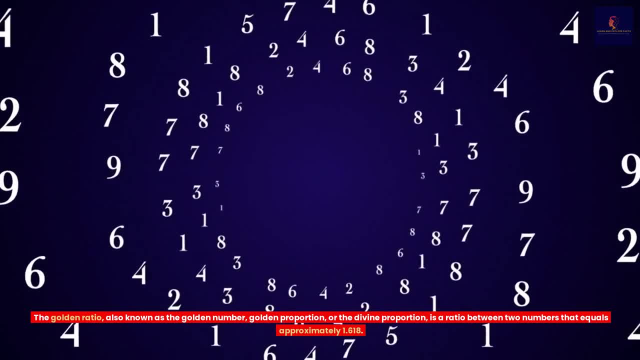 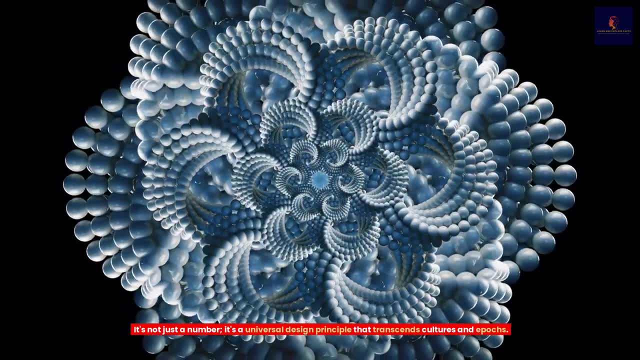 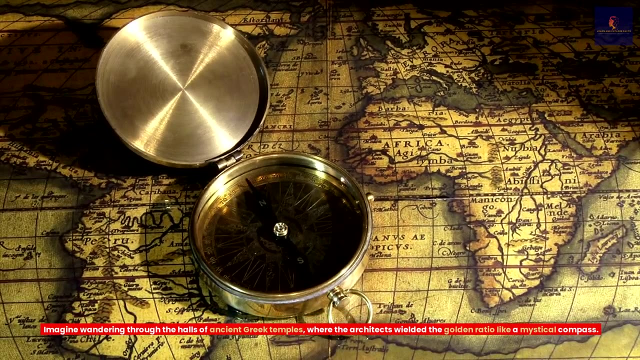 is a ratio between two numbers That equals approximately 1.618.. It's not just a number, it's a universal design principle that transcends cultures and epochs. Imagine wandering through the halls of ancient Greek temples where the architects wielded the golden ratio like a mystical compass: The Parthenon's. 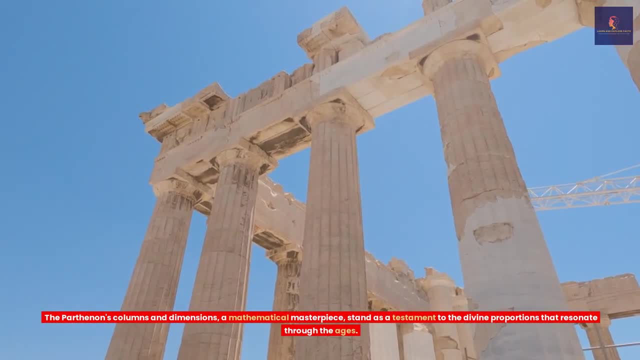 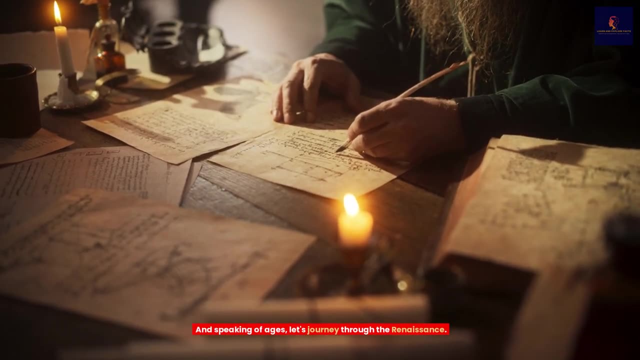 columns and dimensions, a mathematical masterpiece, stand as a testament to the divine proportions that resonate through the ages. And speaking of ages, let's journey through the Renaissance. Picture the artistry of da Vinci, the maestro of the golden ratio, From the Mona Lisa's gaze to 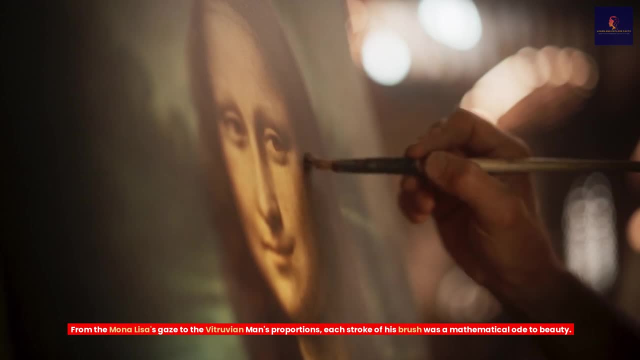 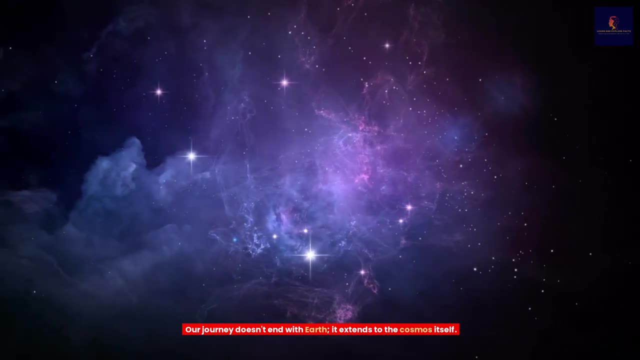 the Vitruvian man's proportions. each stroke of his brush was a mathematical ode to beauty. Our journey doesn't end with Earth. It extends to the cosmos itself. The Fibonacci sequence and the golden ratio aren't mere earthly phenomena. They resonate. 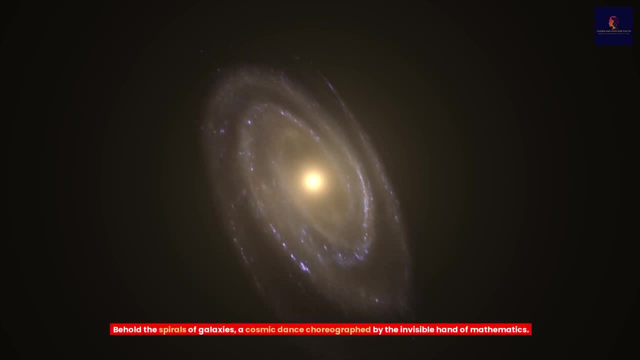 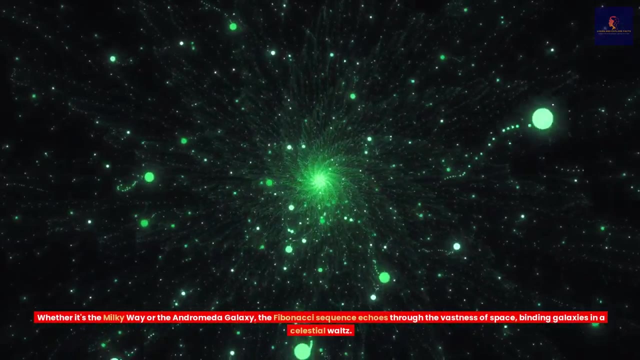 in the grandeur of the universe. Behold the spirals of galaxies, a cosmic dance choreographed by the invisible universe. The universe is a cosmic dance. a cosmic dance, a cosmic dance hand of mathematics, Whether it's the Milky Way or the Andromeda galaxy, the Fibonacci sequence. 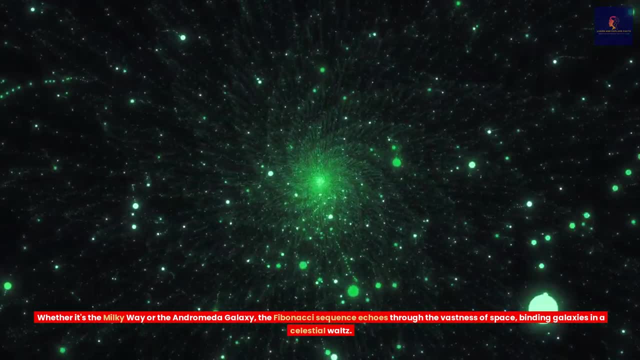 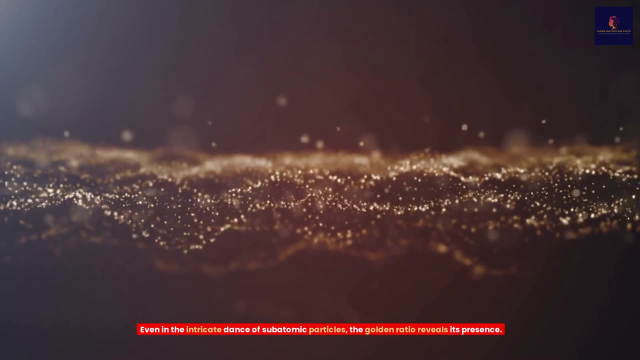 echoes through the vastness of space, binding galaxies in a celestial waltz. Even in the intricate dance of subatomic particles, the golden ratio reveals its presence. It's as if the universe itself is composed like a grand symphony harmonizing with the rhythms of mathematics. 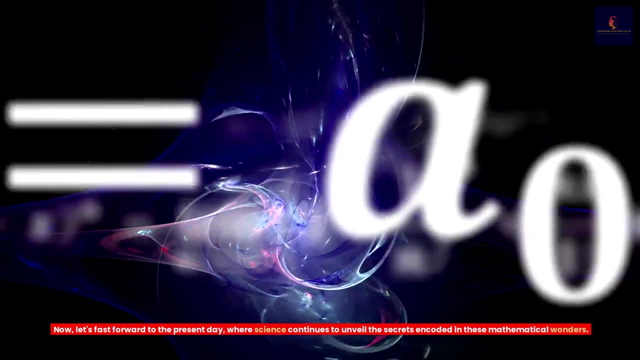 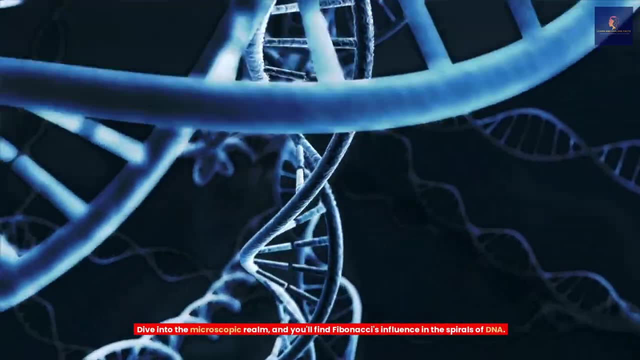 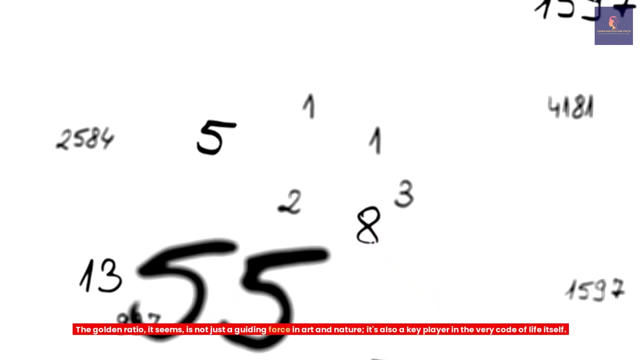 Now let's fast forward to the present day, where science continues to unveil the secrets encoded in these mathematical wonders. Dive into the microscopic realm and you'll find Fibonacci's influence in the spirals of DNA. The golden ratio, it seems, is not just a guiding force in art and